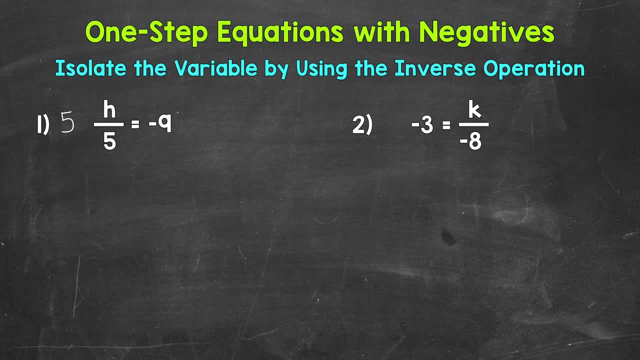 So let's multiply the left side of the equation by 5.. Now, whatever we do to one side of the equation, we must do to the other in order to keep it balanced and equal. Let's multiply the right side of the equation by 5 as well. Now let's take a look at the left side of the equation. 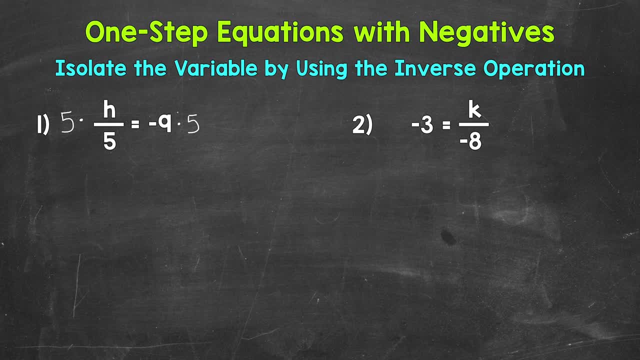 We are dividing by 5 and multiplying by 5.. So these 5s cancel out, They equal 1, because when we multiply h divided by 5 by 5, we end up with 5h over 5.. We have 5 divided by 5, which gives us that 1, and then we have the h We end up with. 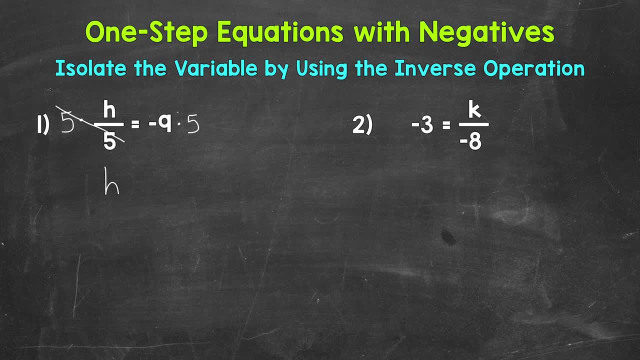 1h, which is just h. Our variable is now isolated. h is by itself, So h equals. and then on the right side of the equation, we have negative 9 times 5. We have a negative times a positive, which equals a negative. So 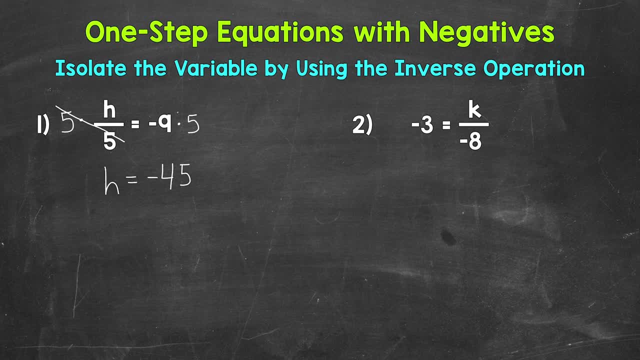 this equals negative 45.. h equals negative 45. That's our solution. Now we can always check a solution by plugging it into the original equation. So let's plug negative 45 in for h, So we have negative 45,. 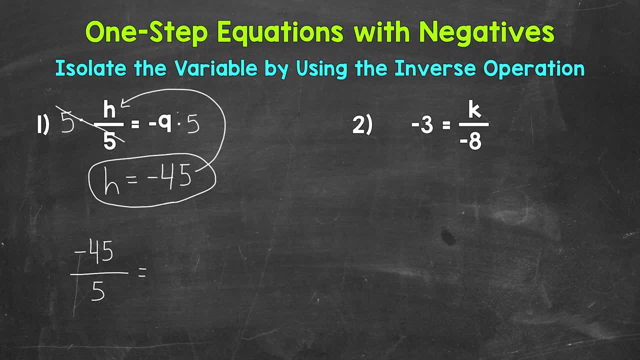 divided by 5, equals negative 9.. We have a negative divided by a positive, Negative 45 divided by a positive 5.. A negative divided by a positive equals a negative Negative. 45 divided by 5 does equal negative 9.. So we have the correct solution: h equals negative 45.. 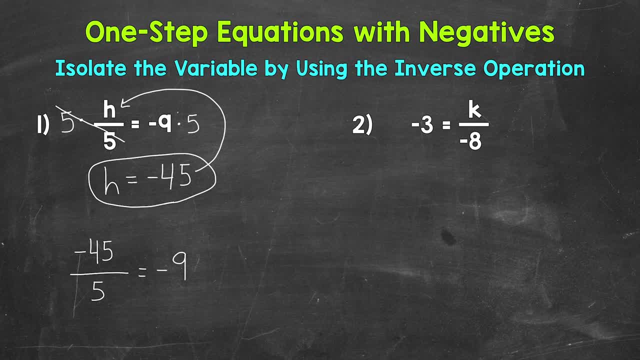 Let's move on to number 2, where we have negative 3, equals k divided by negative 8.. We need to isolate that variable of k. Since k is being divided by negative 8,, we need to undo that division by using the inverse operation.